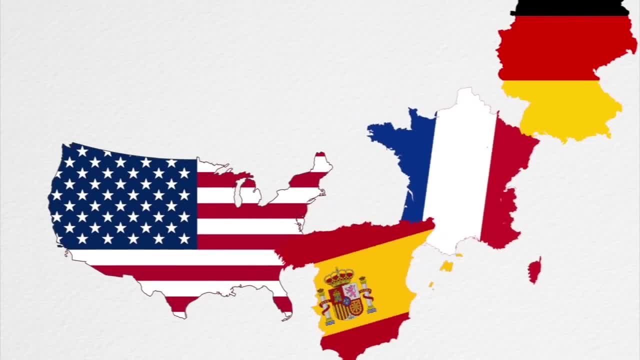 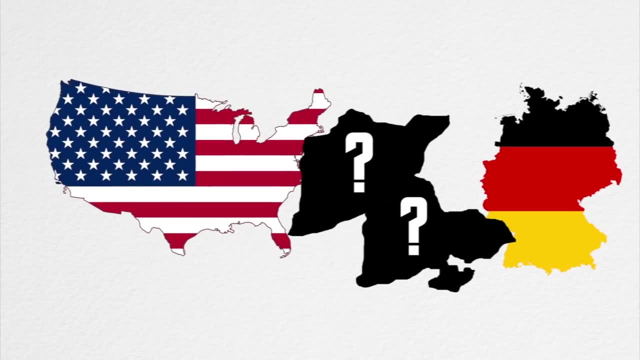 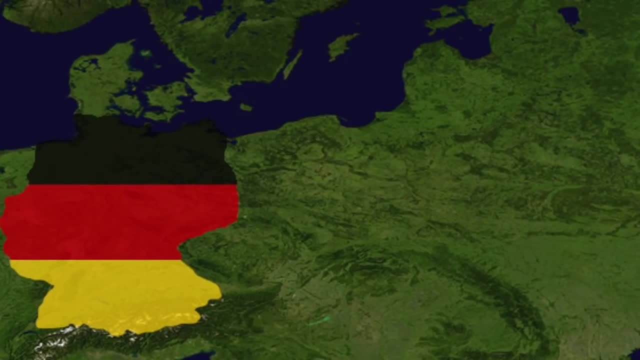 mean France and Spain, once you exclude the Atlantic Ocean. No, What I mean is that Germany borders a country that borders another country that borders the US. Okay, but how Well, let's start in Germany First. you're going to want to go east? Well, actually, as a bit of a spoiler, you're going to want to go east. 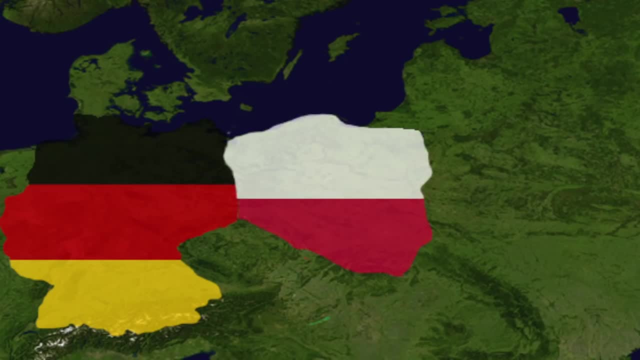 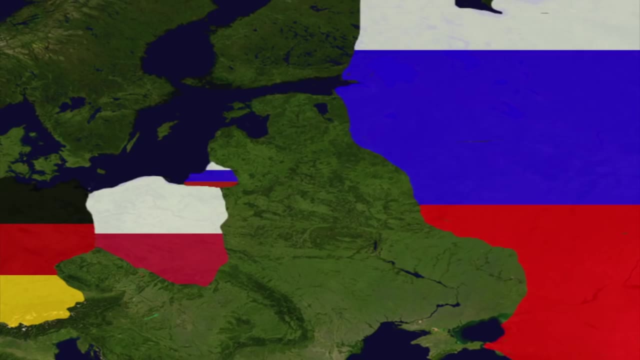 the whole way. So first we reach Poland, which obviously borders Germany, And, as if they hadn't had enough of their bad neighbors, Poland also borders Russia, which is obviously crucial to this. Now, Poland doesn't border Russia proper, but it does border the exclave. 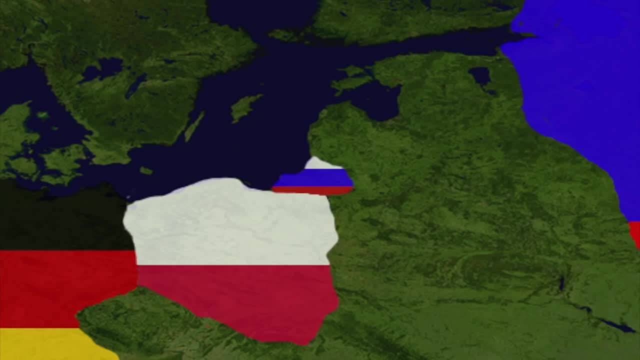 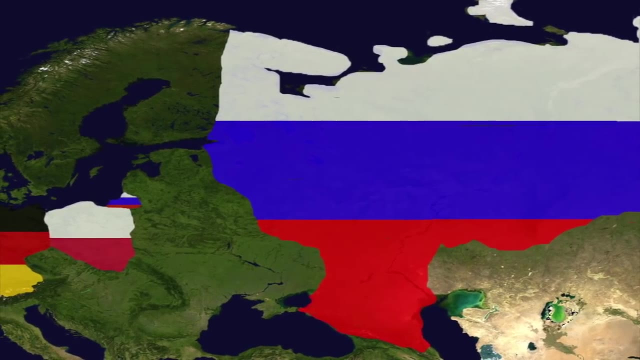 of Kaliningrad, which, I'm sure all the comments will be quick to point out, was once the German city of Königsberg. Now, Russia is, of course, going to help us because it is…. is it too late to say heck and chonker? Yeah, it probably is. I've already made that joke a couple. 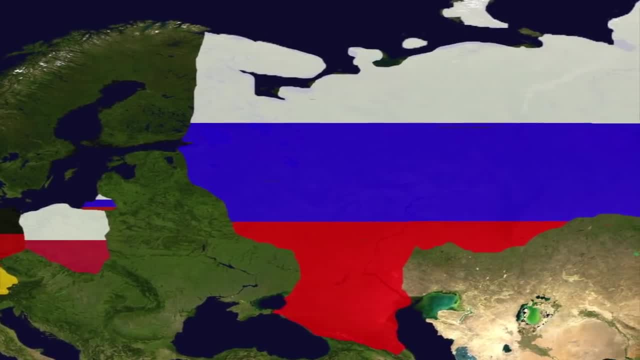 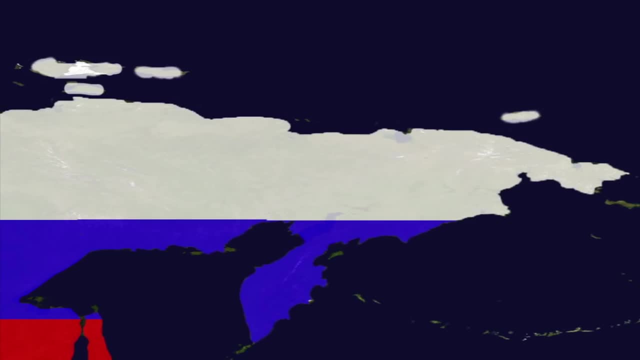 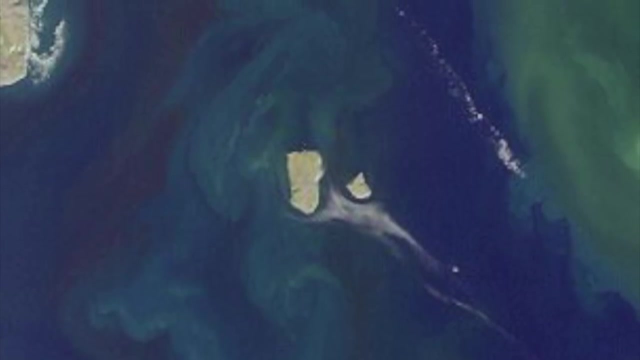 times, But nonetheless, Russia is massive. So, going east, we eventually reach the northeasternmost point in all of Asia, Or actually a little bit east of that, to the Diomede Islands. Now, you've probably heard of these guys. They're a pair of islands, one of which belongs to Russia and the other 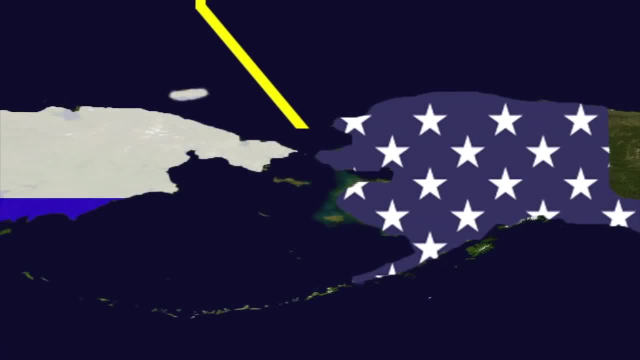 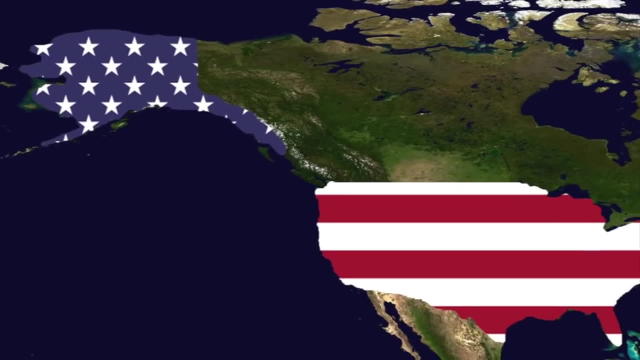 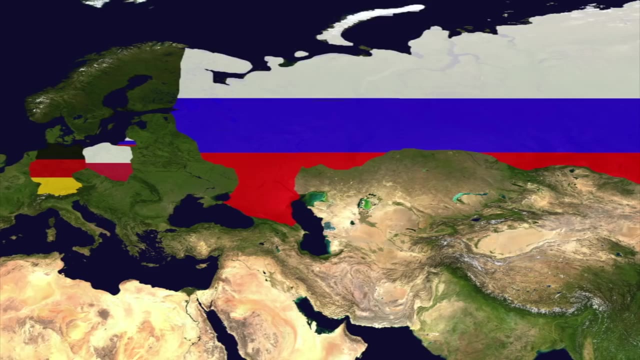 to the US, And right between the two runs a maritime border between Russia and the US, putting two countries border to border directly between the US and Germany. What's crazy about this is that when I said there are only two countries between Germany and the US, 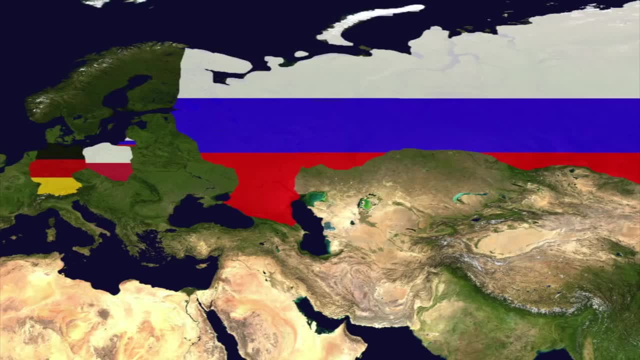 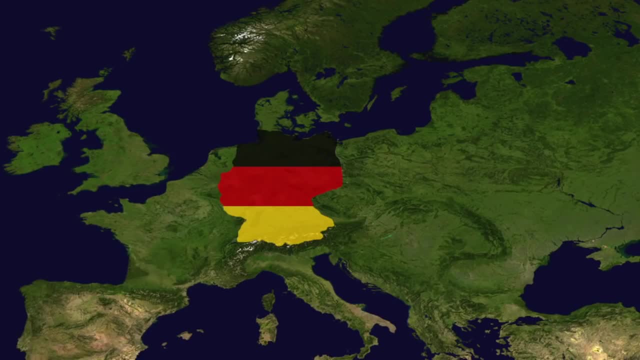 I didn't necessarily have to use Poland and Russia as examples. There are actually two more pairs I could have used, as pointed out on Twitter by Geography World. So what other countries does Germany border? Well, let's see Czechia, Austria, Switzerland…. 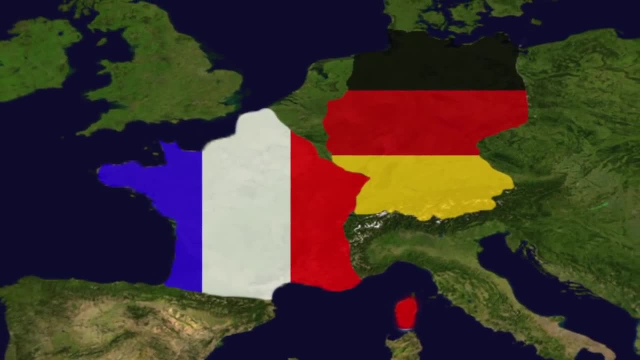 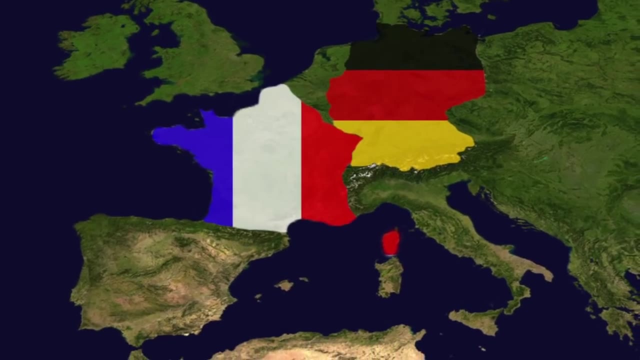 France. France is, somewhat famously, not confined to its territories in mainland Europe and Corsica, but also has far-flung territories scattered all over the place, most of which also fully count as France. And that's all to this. in this video, we're going to be talking about the two most important. 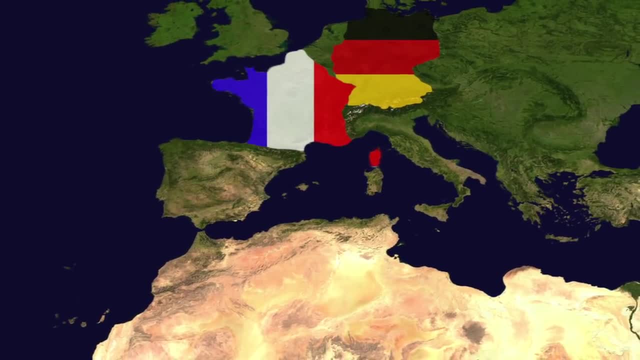 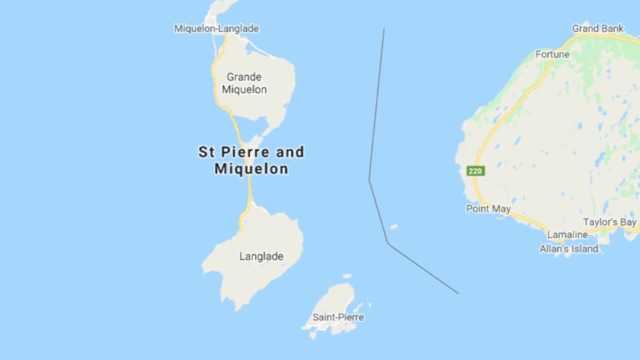 If you want to learn more about these. I made a video on these such territories a few months ago, but what you need to know here is of the existence of Saint-Pierre-et-Miquelon, a pair of islands located right off the coast of Newfoundland, complete with a maritime 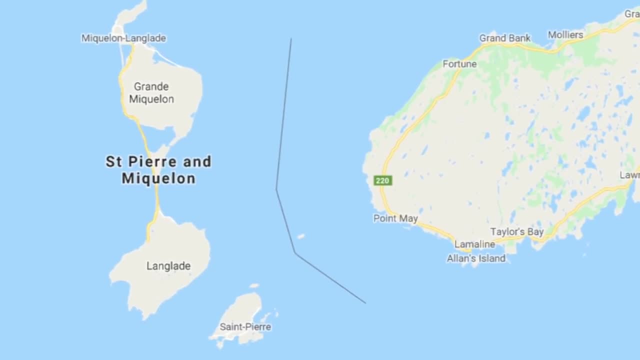 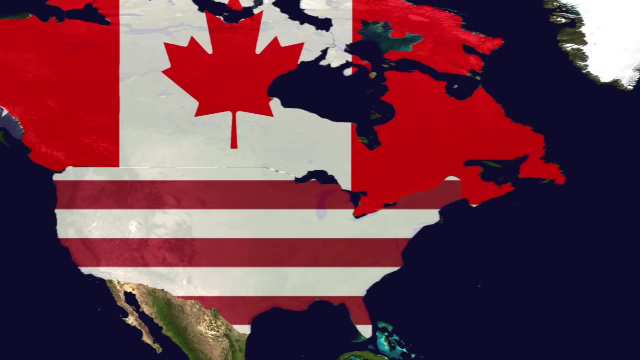 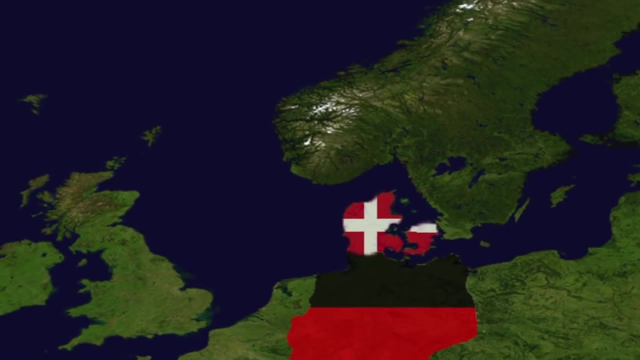 border with the Canadian island. And yeah, we're just going to count maritime borders for the sake of explanation. And now that you're in Canada, yeah, I'm pretty sure Canada borders the US, no problem. finally, we have Luxembourg, Belgium, Netherlands and Denmark. if by Denmark you mean the Kingdom, 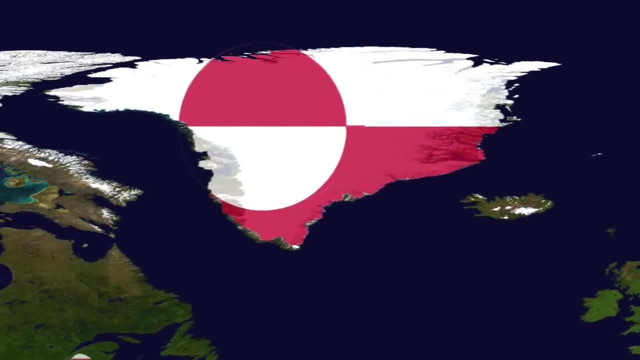 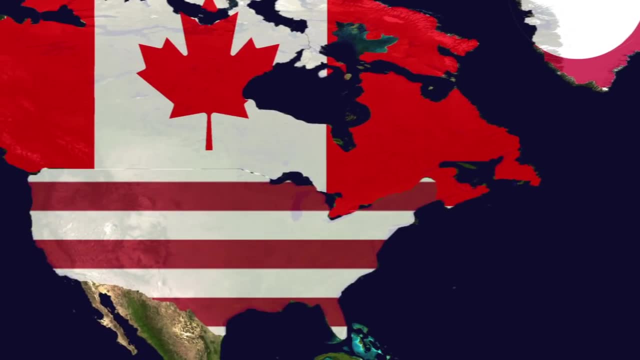 of Denmark, complete with the territory of Greenland, and oh, what's that up there? Oh, you bet that's another maritime border with Canada. need I say more? Okay, maybe not a true maritime border, but it does have a border dispute. 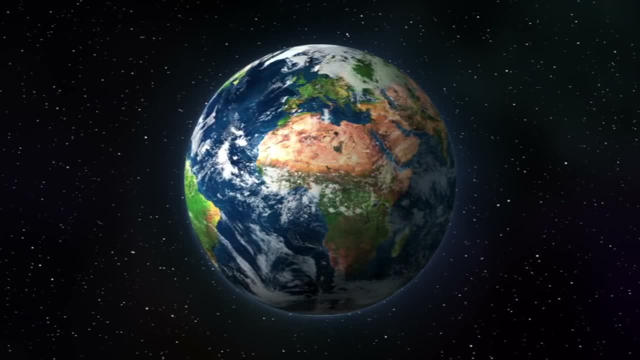 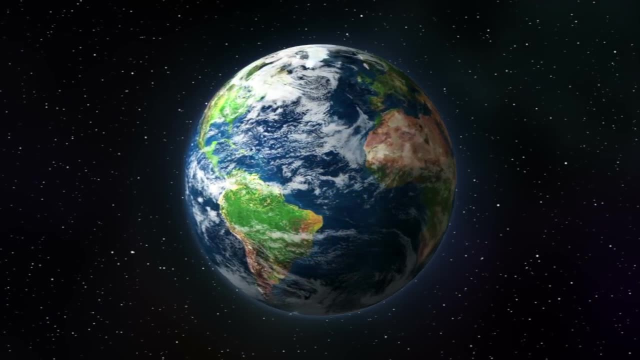 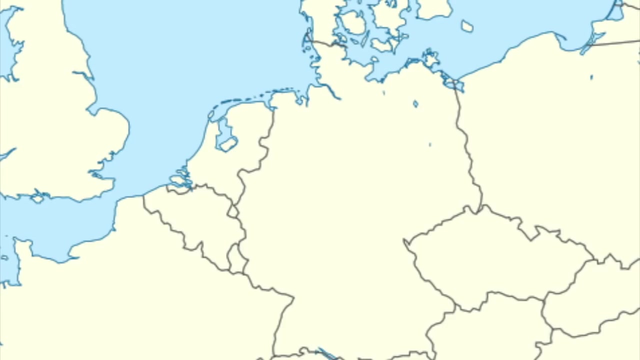 So Germany is two countries away from the US in three different ways. Not exactly a realization that comes intuitively, But one that shows both how big Russia is and how many territories countries like France and Denmark have all around the world. Going back to Germany, a good amount of playing with the measure tool on Google Maps reveals 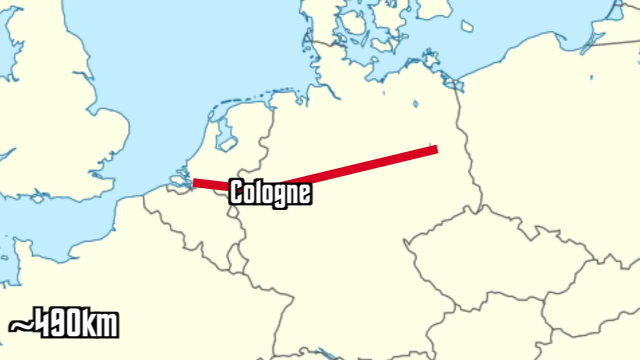 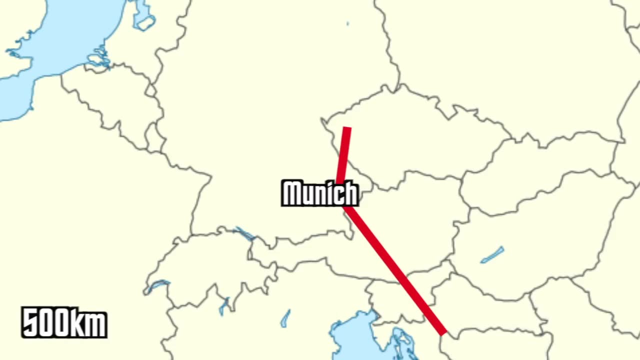 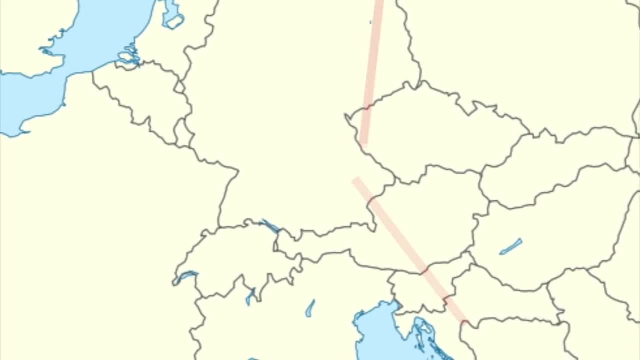 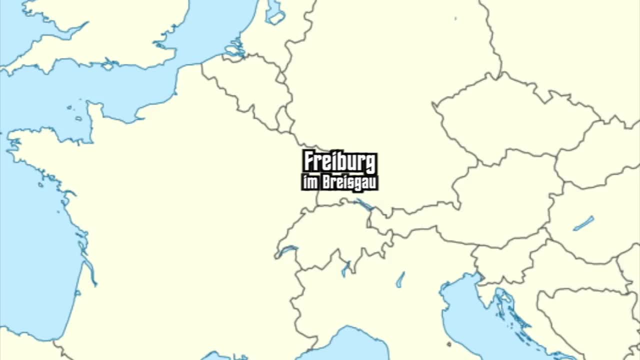 it's kind of a random example really shows how weirdly located Berlin is for a capital, since Freiburg is actually closer to Paris, Brussels, Luxembourg city, Amsterdam, Bern, Ljubljana, Monaco, Liechtenstein, San Marino and even Prague than it is to Berlin. 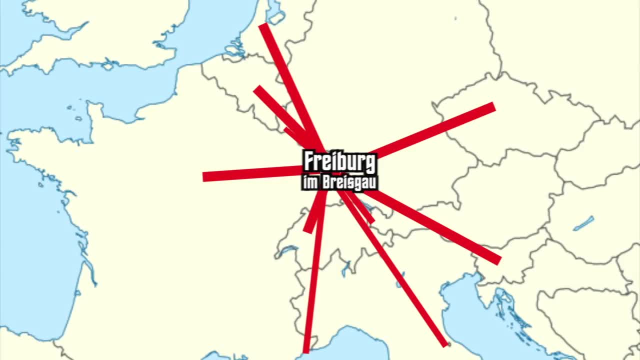 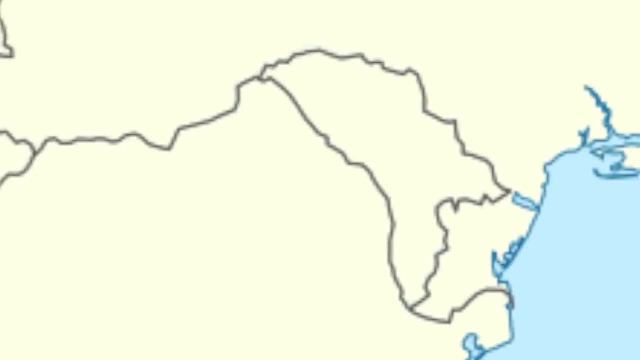 So this is a very strange comparison, because if you take a look around the city, you can. That's 7 foreign capitals. These facts might make you feel like you're this close to losing it, but Moldova is already that close to not being landlocked. 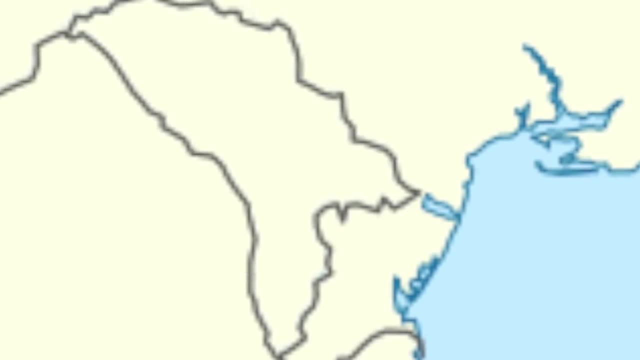 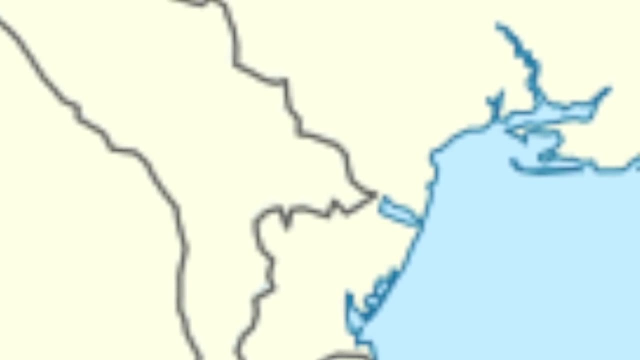 Seriously. the town of Polanka, located about 45 kilometers west of Odessa, is less than 3 kilometers from the Dniester estuary on the Black Sea, But that 3 kilometers of land still belongs to Ukraine. so sorry, Moldova. 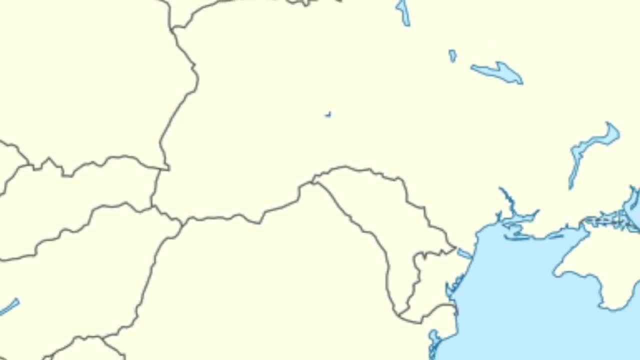 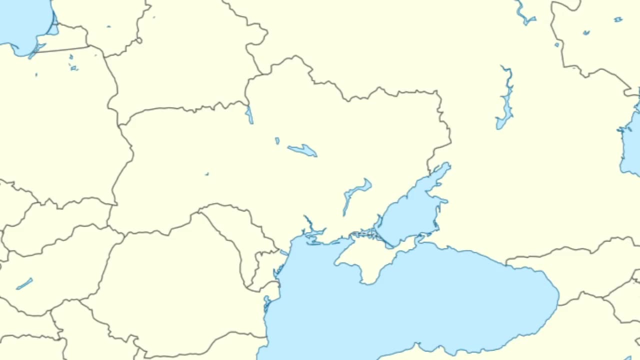 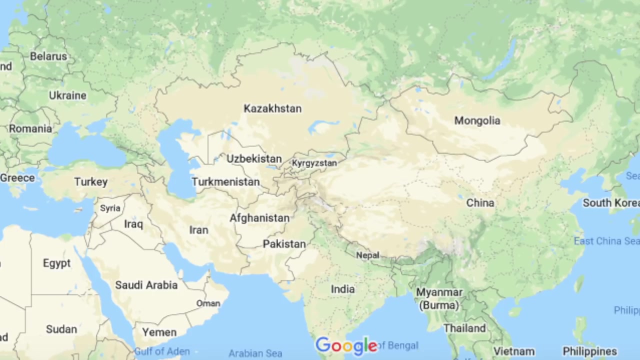 Of course, the countries of Europe themselves are pretty small. Even the largest non-Russian country in Europe, Ukraine, is still smaller than the largest US state. One country that is absolutely ginormous, however, is China. China has always been viewed as being far from Europe and, to be fair, it is, but if 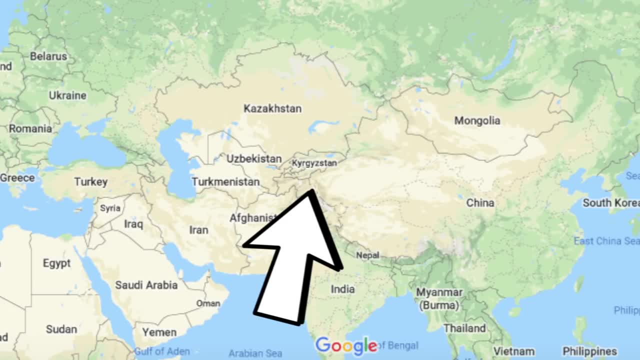 you look at the westernmost point in the country, just west of Kashgar, you'll find that it is actually closer to Istanbul than it is to Shanghai. In fact, it is also close. It's even closer to Belarus than it is to Beijing. 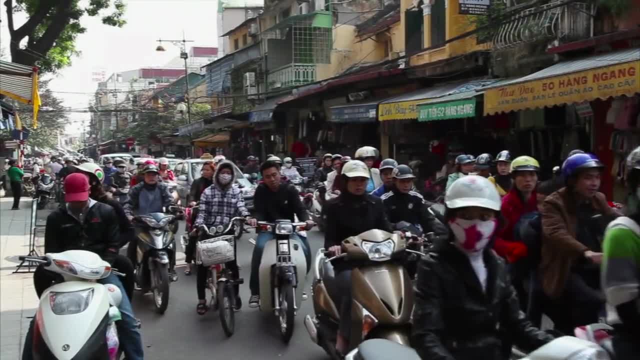 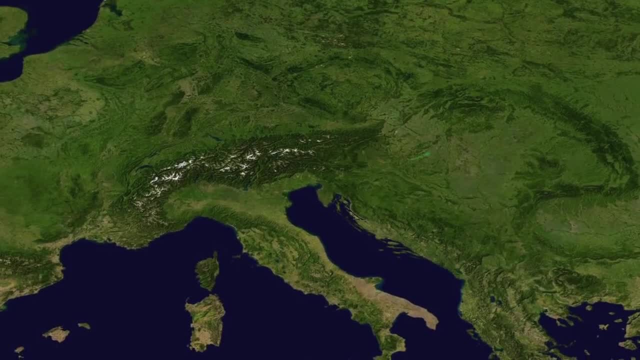 Let's close this video with some fun facts about linguistic geography, as in the geography of where people speak different languages. For instance, what is the closest English-speaking country to Italy? I'll give you a hint: it's a left-side driving island nation. 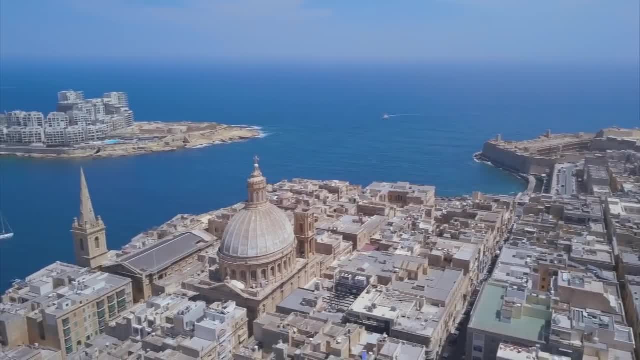 That's right, it's Malta. And well, to be fair, they were a British colony at one point, so that would explain that. Finally, what is the largest English-speaking country in the world? I'll give you a hint: it's Malta. 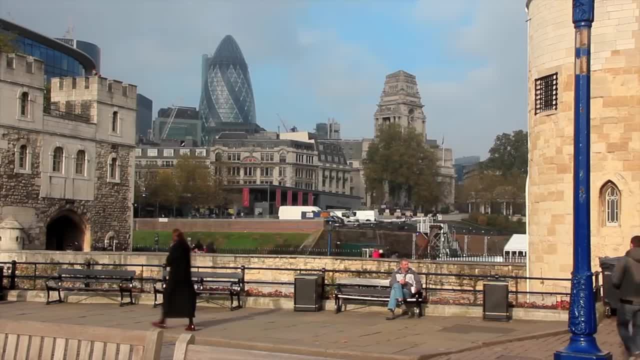 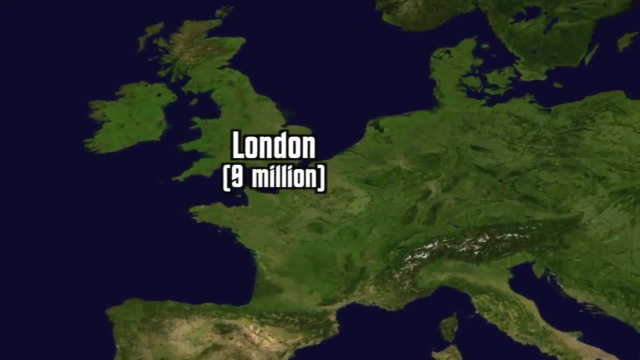 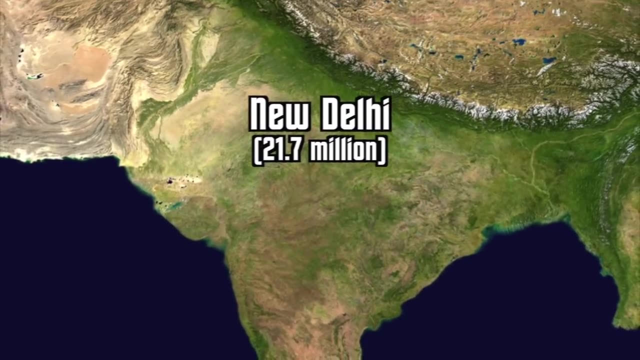 By that I mean what is the most populous city in an English-speaking country? It's not New York, it's not London, it's not even in what's generally considered the Anglosphere. It's New Delhi, India, home to roughly the same number of people as live in New York. 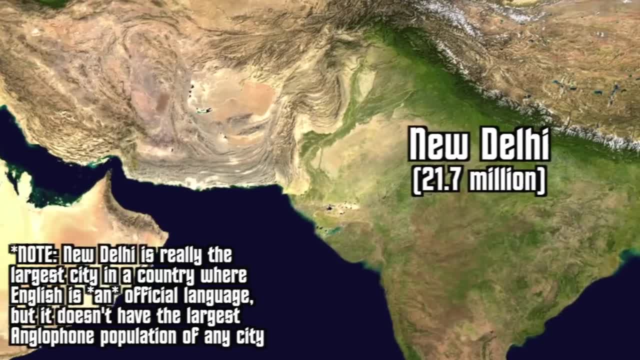 and London Combined. Okay, now, what is the largest Francophone city in the world? Judging from the last answer, of course, I'm guessing you're waiting for me to answer. I'm guessing you're waiting for me to answer this one. 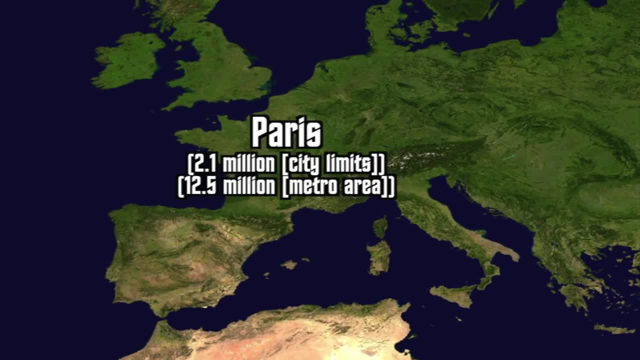 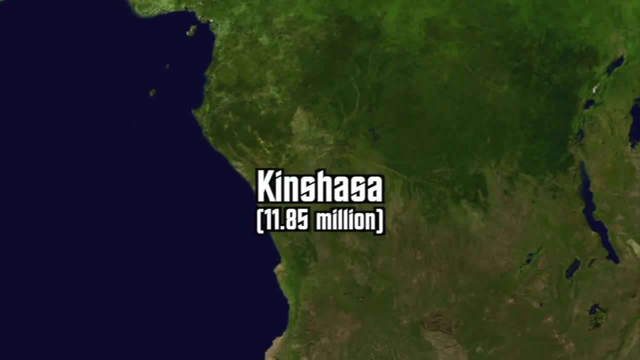 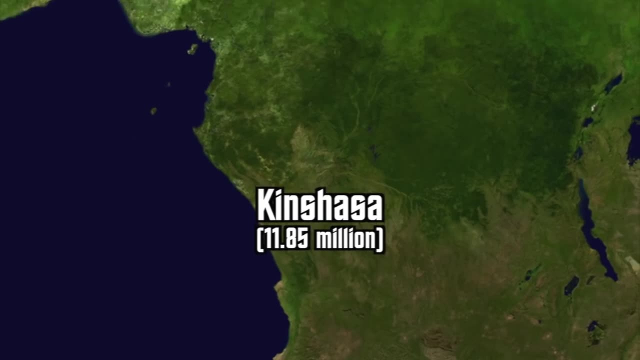 I didn't say Paris. I didn't say Paris, And you're right. it's not Paris, It's Kinshasa in the Democratic Republic of the Congo. Lastly, what is the largest German-speaking city in the world? This is a bit of a tough one, isn't it? 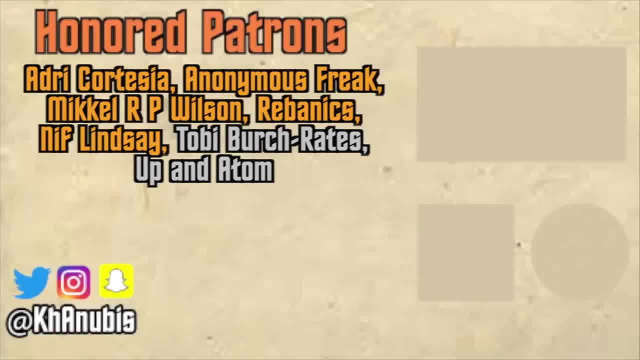 Yep, okay, it's actually Berlin. the world isn't that weird, As always. thanks for watching and please let me know if you want more of these videos in the future, If you want to peer in on discussions about future videos, memes and other random stuff. 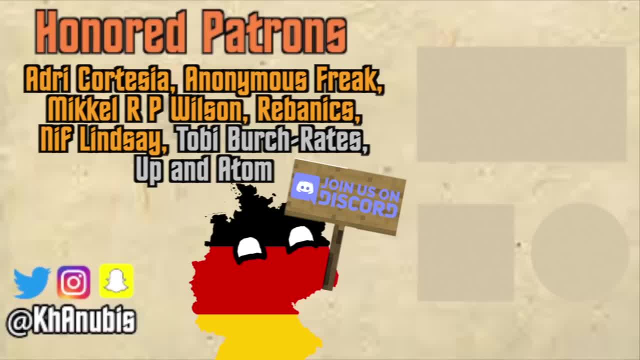 Be sure to join the Discord server and also please be sure to like, share and subscribe to learn something new every Sunday.